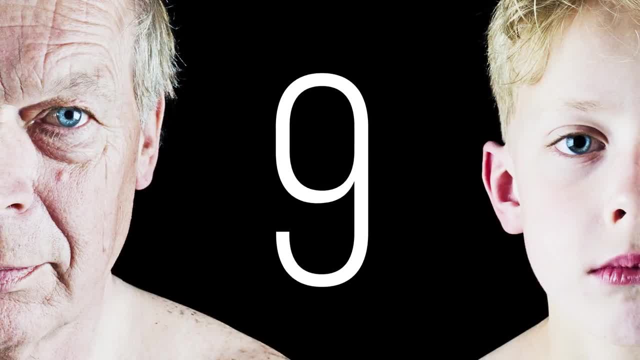 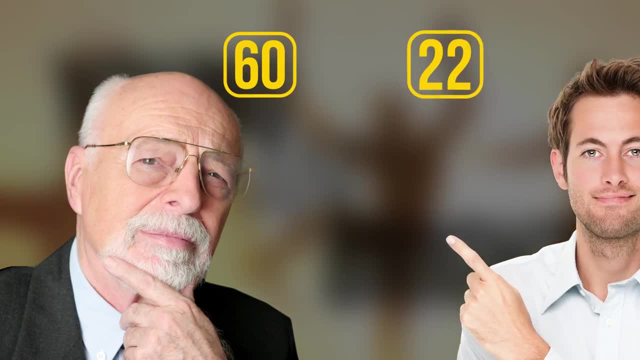 If you get 9 as your mental age, it does not mean your IQ is low. It only shows your perception of the world is young and bright. If you get 60 while you're 22,, it's not too bad either. It just means 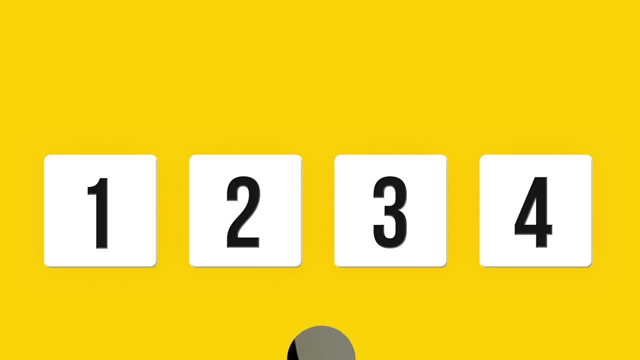 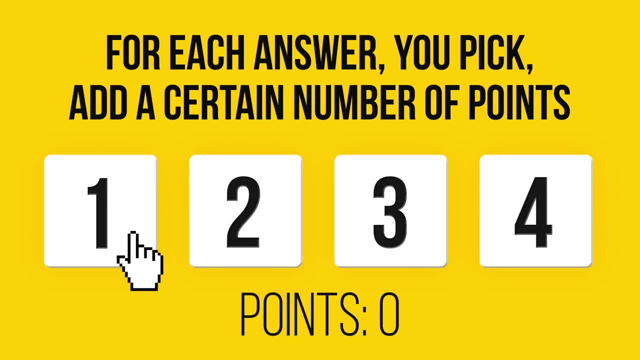 It just means you are really wise. For each answer you pick, add a certain number of points. You get one point. for each time you choose number one option, You get two points for option number two, And so on. There will be four options for each question. 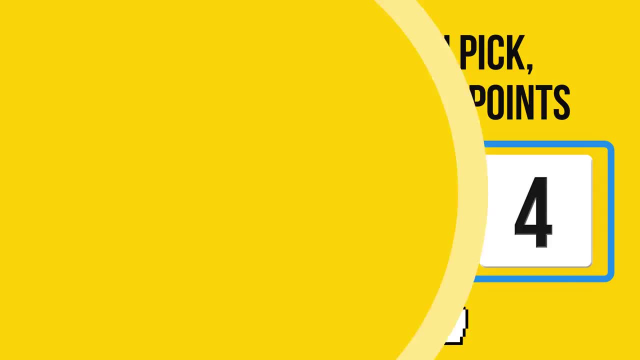 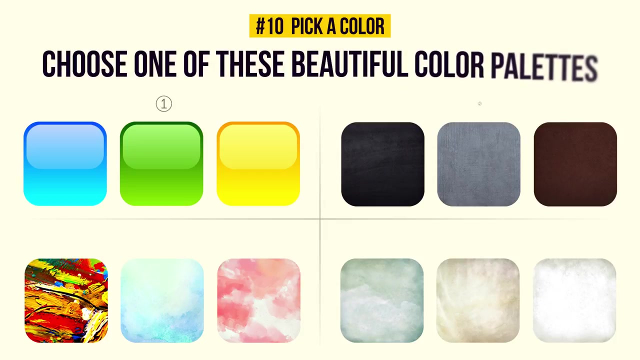 Let's get it started in here. Starting with number 10, pick a color. The first question is as easy as can be. All we want you to do is choose one of these beautiful color palettes, Really, whichever you like most. when you just saw all the options, go for it. 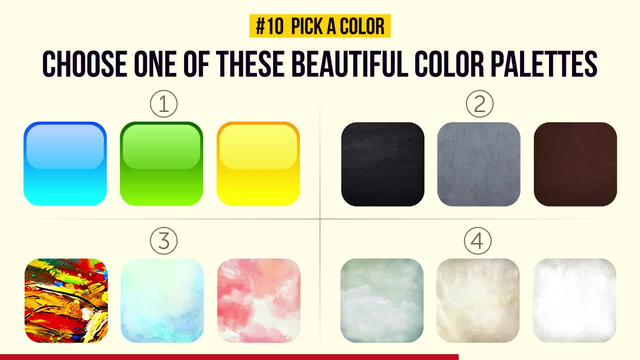 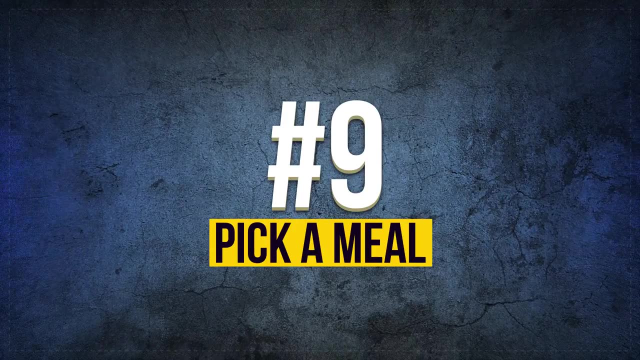 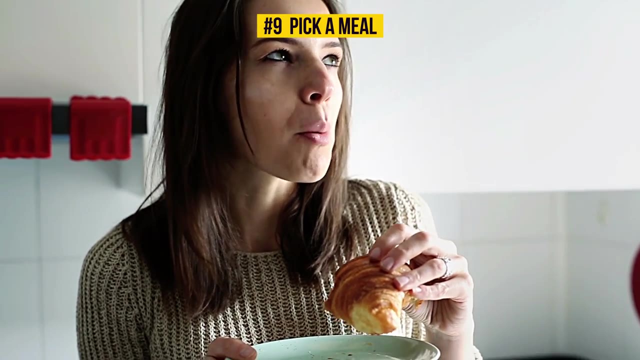 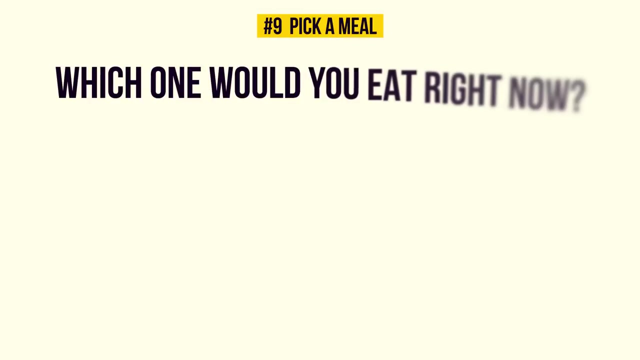 Number 9. Pick a meal If you're hungry. we're sorry for this one, but it is an important part of the test Plus, that food looks so good. If you could pick any of these meals, which one would you eat right now? 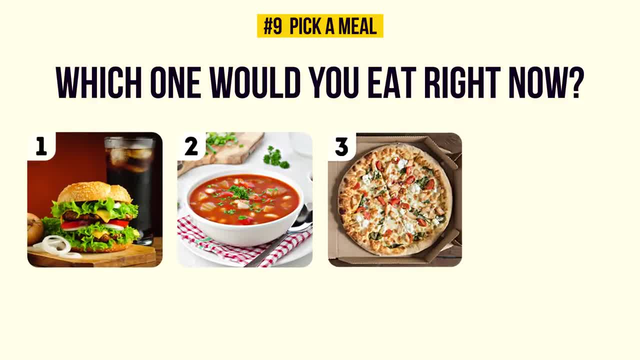 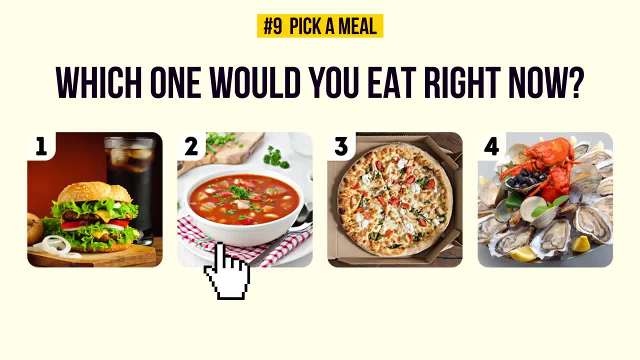 1. Hamburger, 2. Soup, 3. Pizza, 4. Seafood, A juicy steak, crispy bread straight from the oven. Will you pick the hamburger? But then again, your mom always told you how important it is to have enough soup. 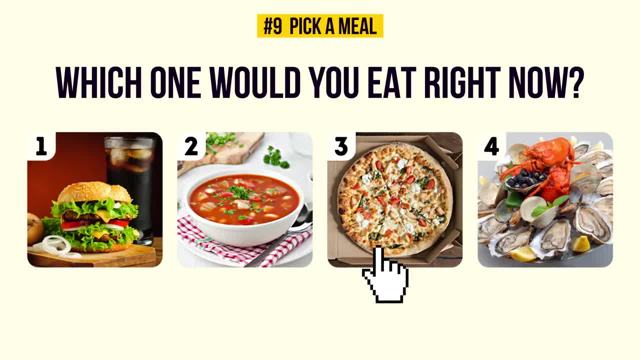 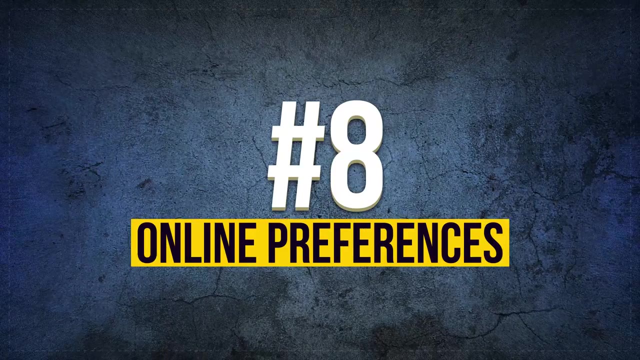 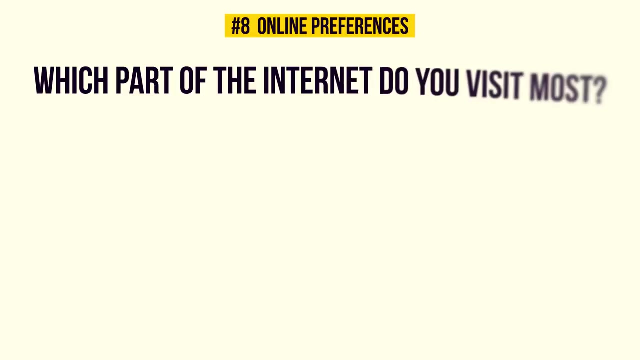 Nutritious and warming up. Or will you go for the pizza? It needs no introduction. Fancy enough to choose seafood? Eh, it's up to you. Number 8.. Online preferences: Which part of the Internet do you visit most? 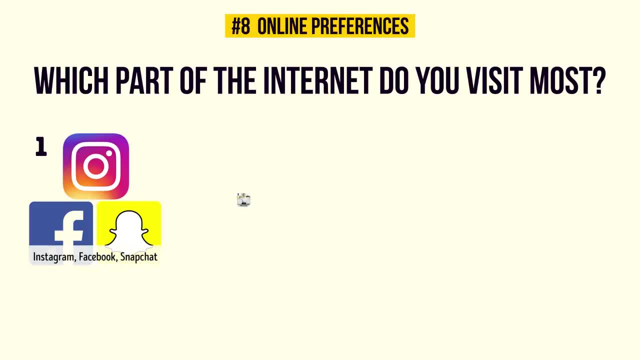 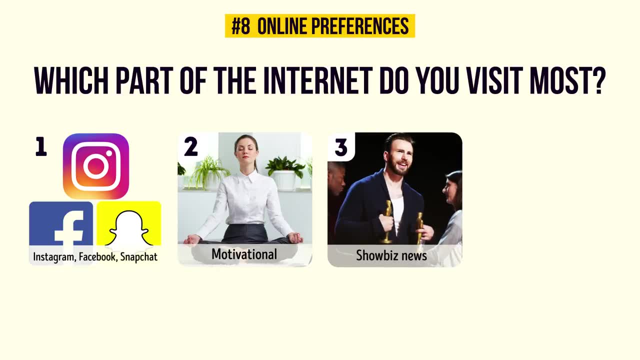 1. Instagram, Facebook, Snapchat. 2. News sources, motivational and time management websites. 3. Celebrity gossip and showbiz news. funny cat videos. 4. I'm not sure how the Internet works, but I check my email sometimes. 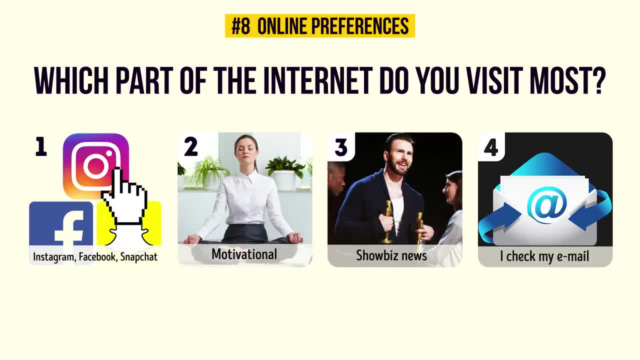 If Instagram means the world to you, pick option 1.. You care a lot about getting more efficient and not wasting a second of life, and you must be interested. If you want to be in the know when it comes to world news, then go with a 2.. 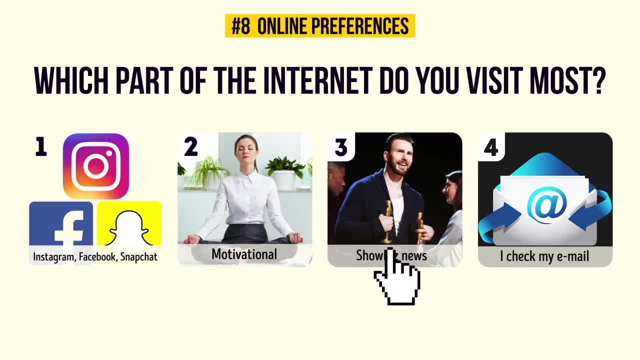 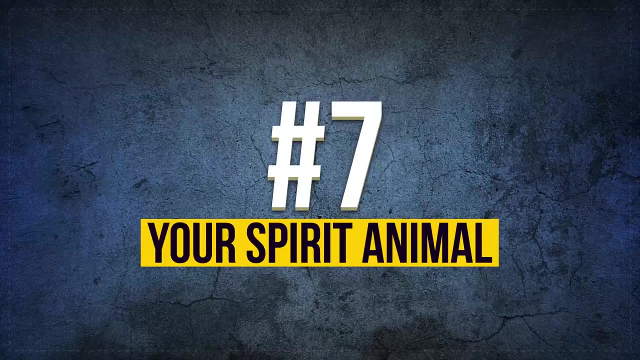 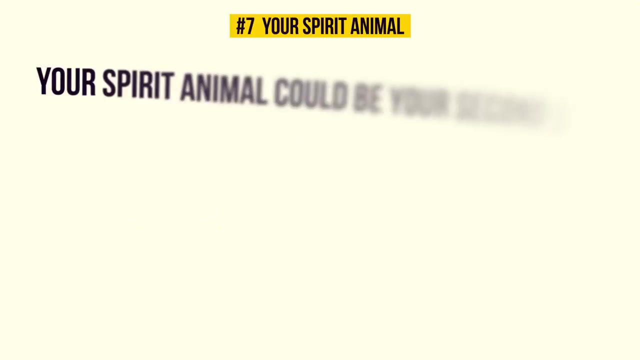 Hey, who cares about politics and nuclear disarmament? Give me some celebrity gossip. You get it if you pick 3. Option 4 speaks for itself. 5. Number 7. Your spirit, Your spirit animal, could be your second self. so pick wisely. 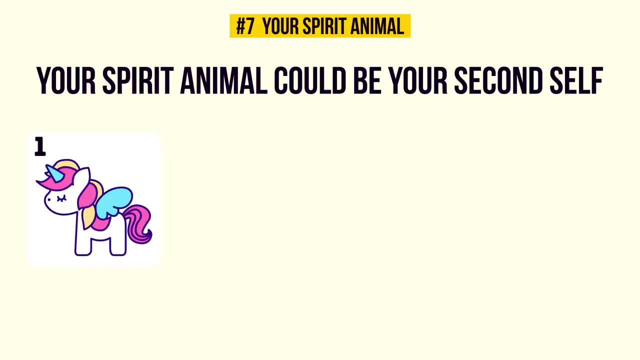 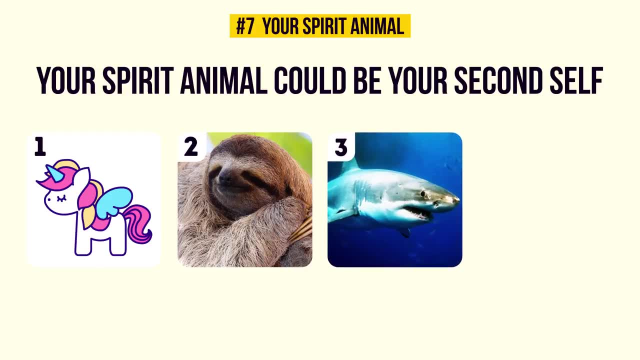 Is it going to be Number 1. Unicorn, Magical, wild and free Ooh. Number 2. Sloth- Need I say more? Number 3. Shark: Determined and dangerous. Or 4. Who needs a spirit animal? 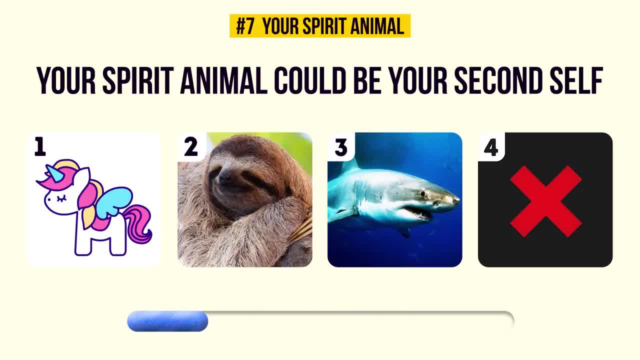 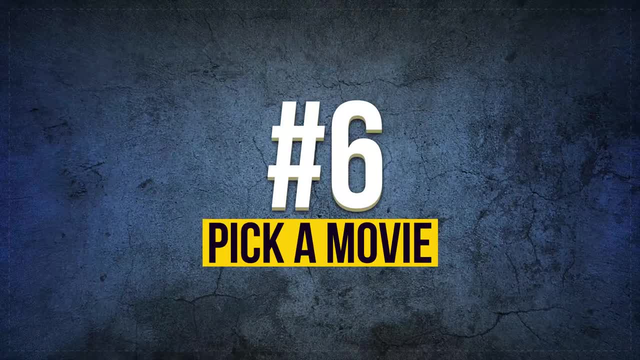 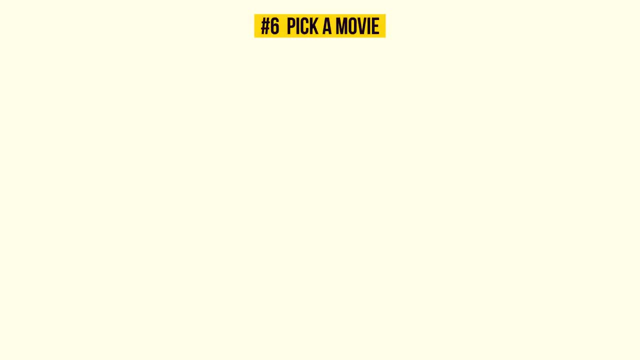 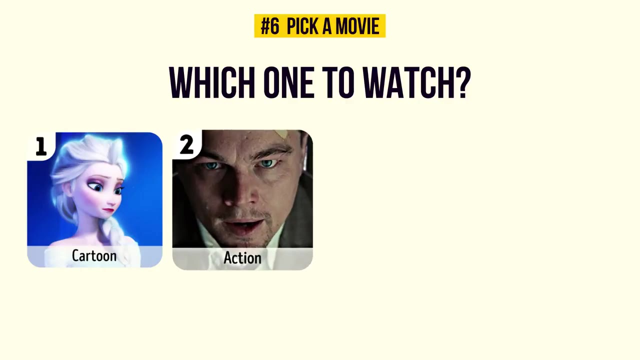 Question 5.. Question 6. Pick a movie. It's movie night and you get to choose which one to watch. What'll it be? 1. A cartoon or family movie? 2. Action, fantasy or horror? 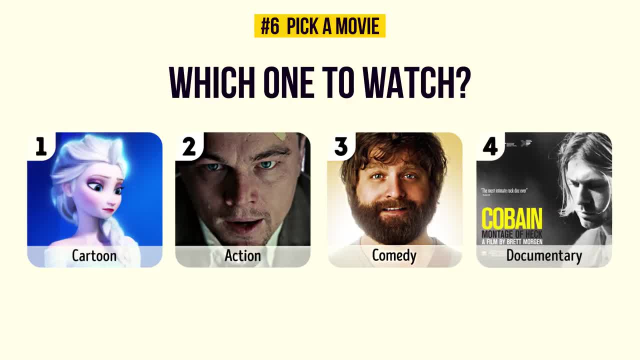 3. A good old comedy. 4. drama, romantic drama or documentary. Now, if Frozen makes your heart melt, breaking every common-sense rule, or if you're still laughing at the adventures of Home Alone Guy, go for option 1.. 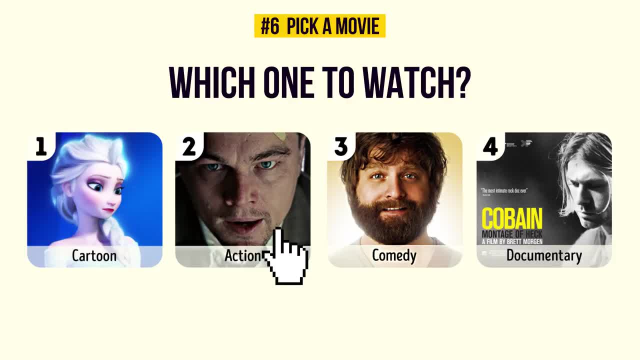 For those who like to be terrified or thrilled with action, number 2 is waiting for you. In case you are a hangover type of person, we mean when it comes to the movies- there is option 3 right there, Crying over the notebook. 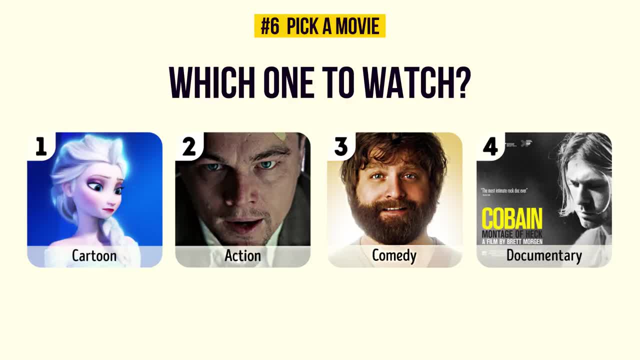 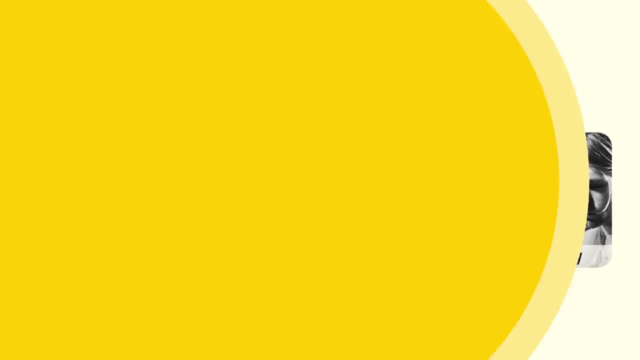 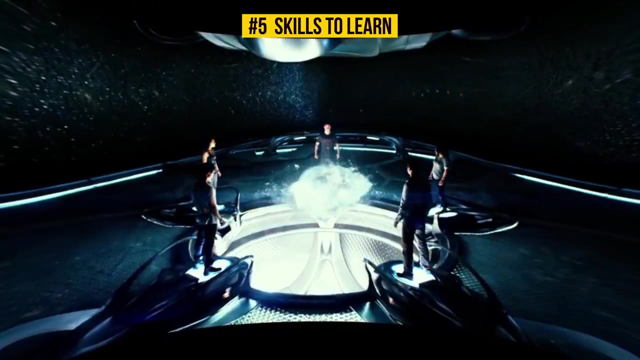 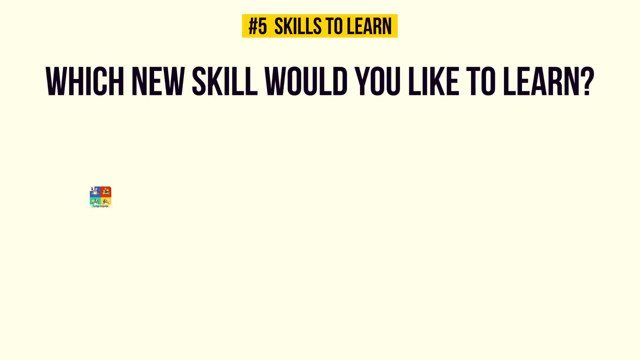 Go for option 4.. And do you have a tissue Question? 5. Skills to learn. Imagine you can pick a skill to learn with no effort, like right now. What skill would it be? 1. Foreign language. 2. Some sports. 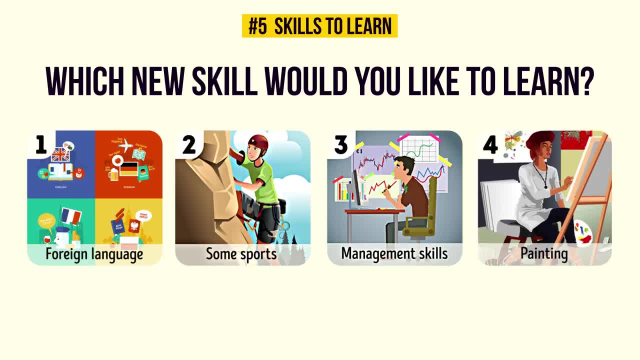 3. Management skills Or 4. Painting. Eh, this is kind of unfair. All the options are so good, But still one must be better for you than the others. Think of all the traveling you can do when you learn to sprechen Deutsch. 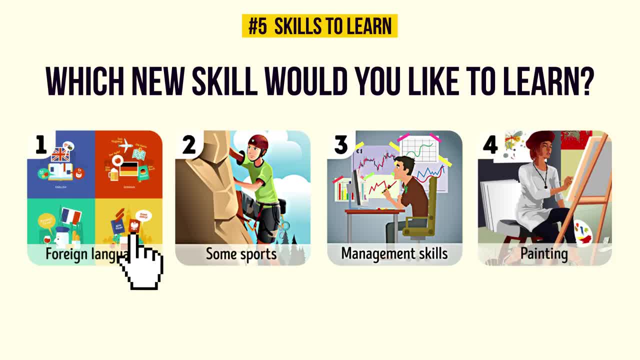 or hey, talk like a New Yorker. It's a language. Or how fit your body will get and how much cooler you will become when you master basketball, or maybe alpine skiing, Or 3. An amazing bide. 4. The three most important things when you learn German are: 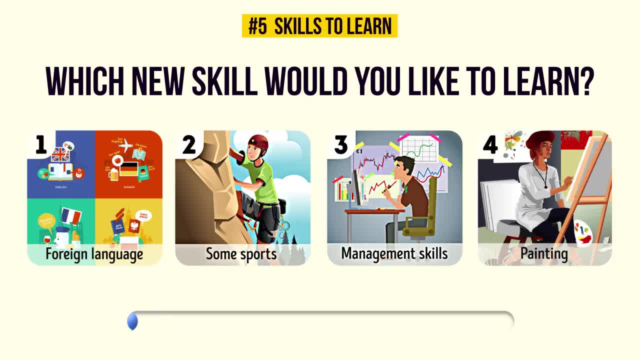 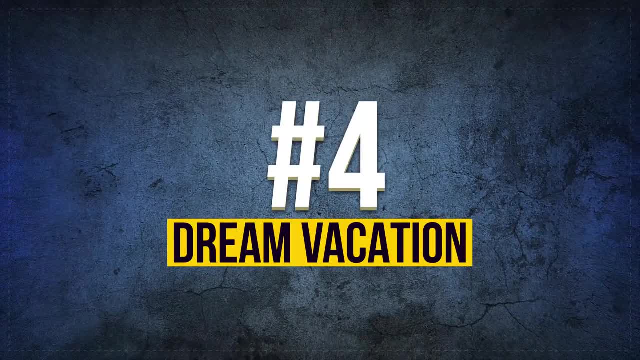 1. The language, 2. The language, 3. The language, 4. The language, 5. The language, 6. The language, 7. The language. Question 4. Dream vacation. Do you want to go on vacation? 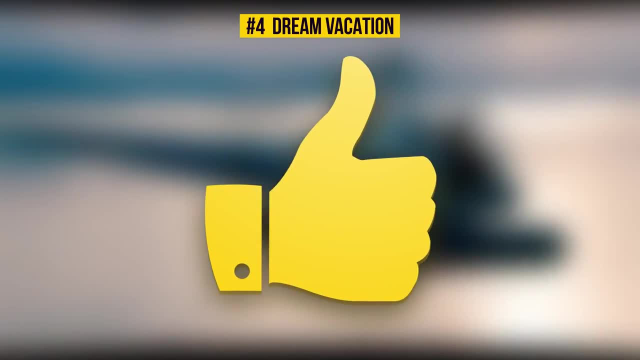 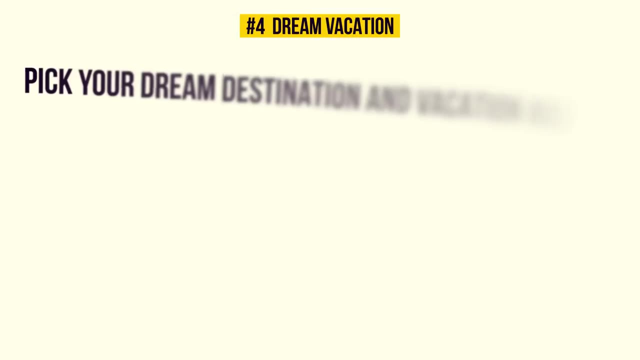 Like right about now. Hit the magical like button. It should get you there. Um, are you still there? Okay, it'll work next time, Trust me. Anyway, pick your dream destination and vacation routine Number one: Disney World. 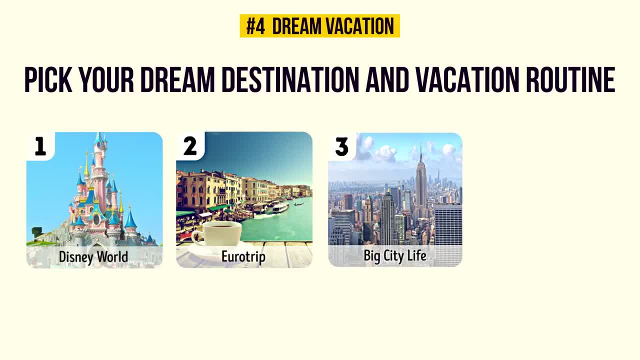 Number two: Eurotrip. Number three: Big City Life. Number four: relax. Take it easy. Imagine all the rides at Disney World. Are you screaming with excitement? Then number one is your best bet. But then again exploring Europe. 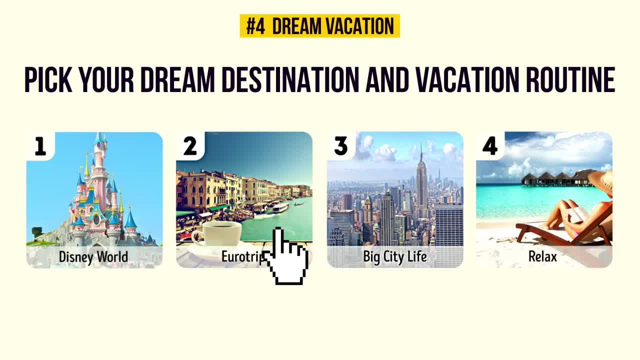 You're with your friends, including its bars and nightlife. Sounds like a bunch of fun: Hitchhiking from romantic Paris to fairy-tale-ish Germany and then to Italy. Ooh dreamy If you're a Big City Life type of person. 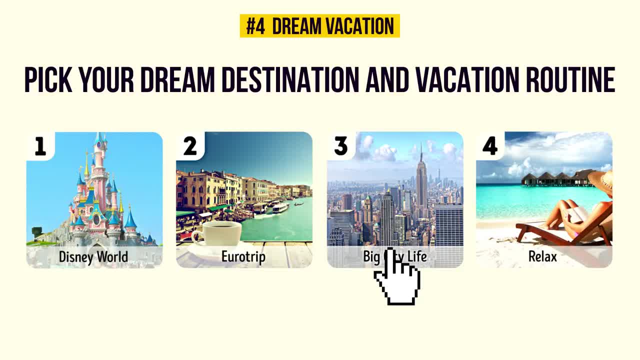 you can choose to discover New York or any other megalopolis Sites, arts and good food everywhere. Number four is an option to escape from the world and all its hustle and bustle: A tropical island or a cottage in the woods. 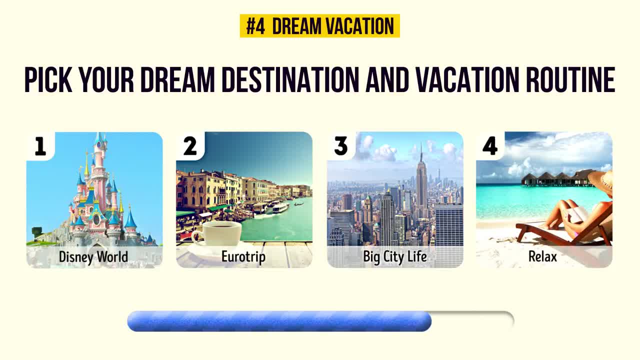 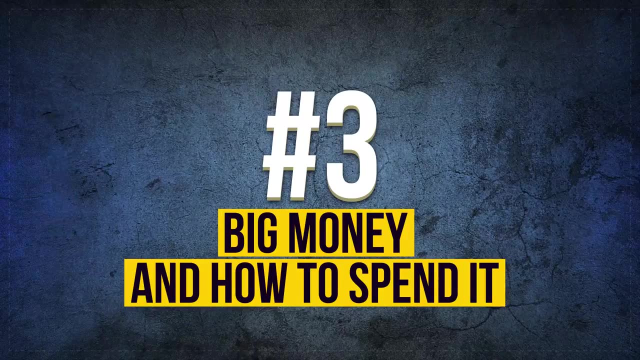 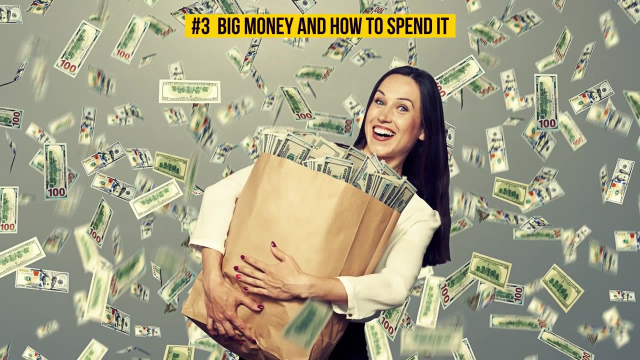 You name it. Question three: Big money And how to spend it. Imagine you have won the lottery. The money is really good and you have four options as to how to spend it. Will you choose to one party it up? 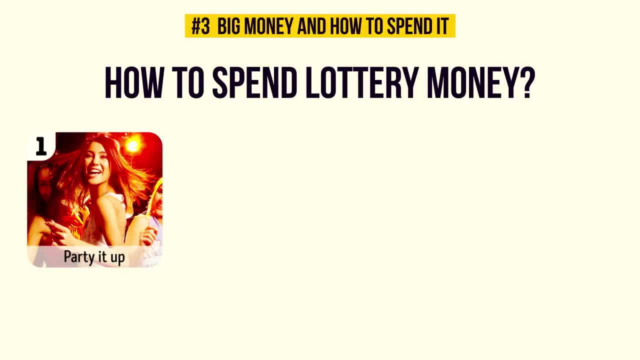 travel the world and buy that Chanel bag you've always wanted. Number two: spend some of it to buy gifts for my loved ones. do a house renovation. Three: use it to pay off the bills and that student loan, Oh yeah. 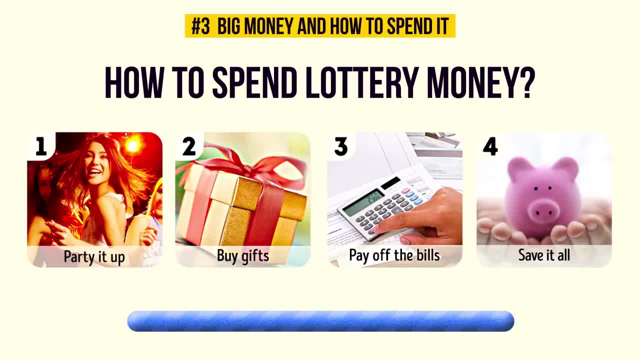 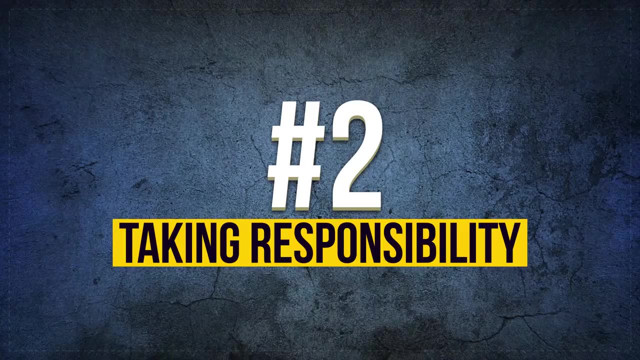 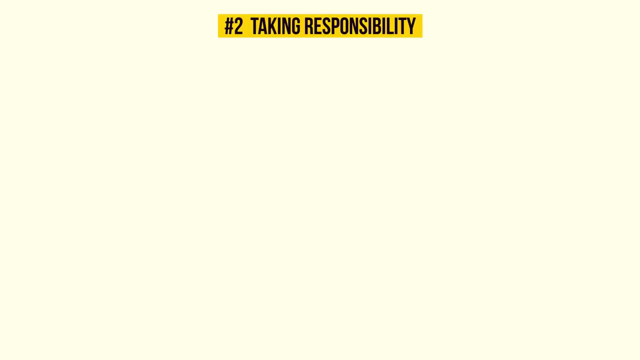 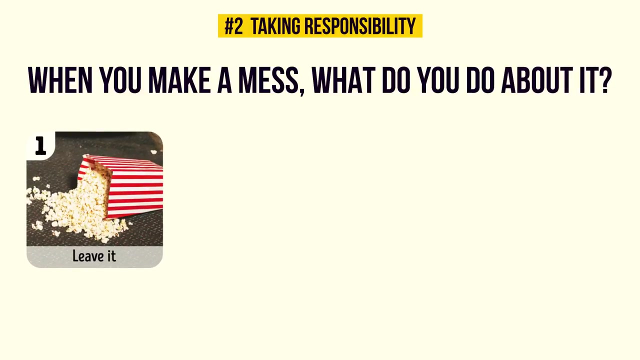 And four: save it all for my offspring. Question two: Taking responsibility. Now be honest with this one. When you make a mess, what do you do about it? One: leave it, Someone else will take care of it. Two: offer to clean it, hoping to hear a no. 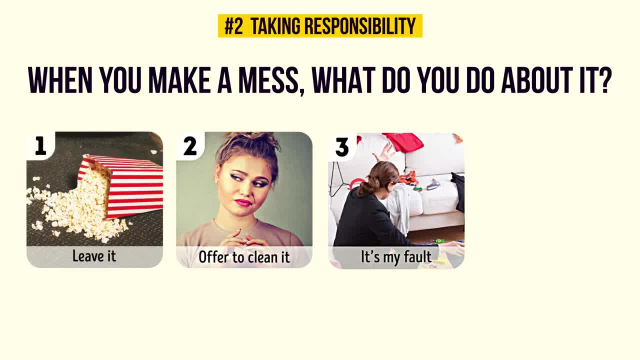 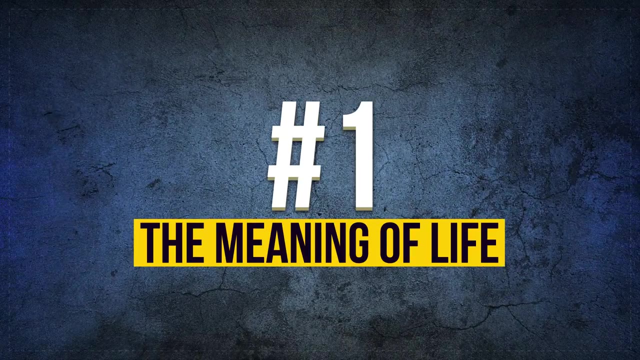 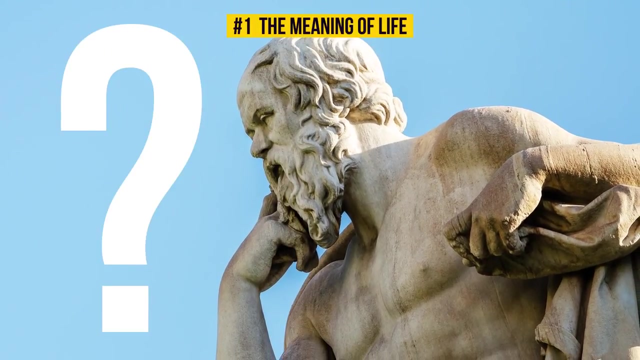 Three silently clean it. It's my fault, after all. Four silently clean it because who else will do it? And finally, question number one: The meaning of life. So what's the meaning of life? That's a philosophical one, we know. 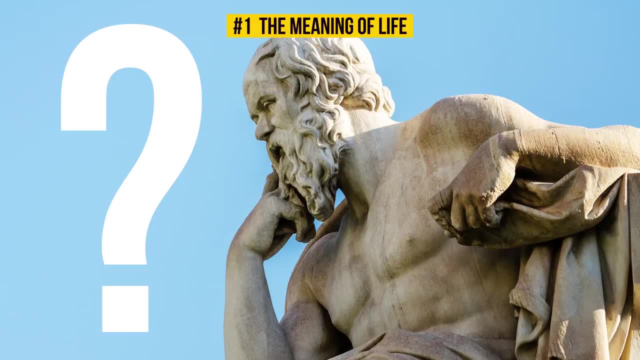 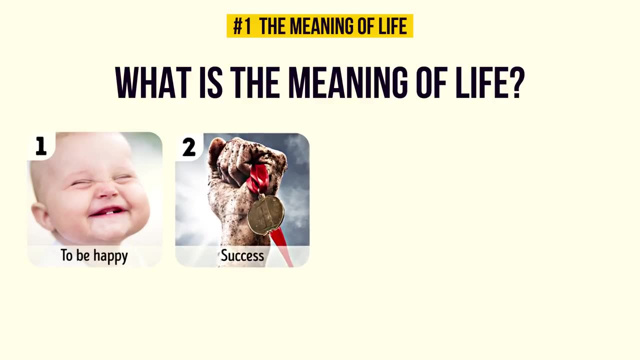 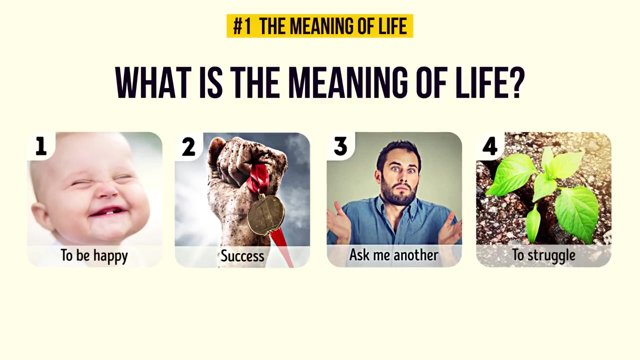 But what did you expect the grand finale to be? Pick an option which seems to be the right one at the moment. Number one: to be happy. Number two: it is the stairway to success. Number three: ask me another. Number four: to struggle. 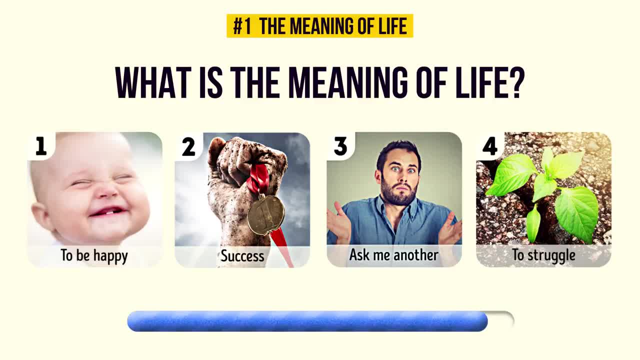 That is the meaning of life. Number five to be happy. Number six to be happy. Number seven to be happy. Number eight to be happy. Number nine to be happy. Number ten to be happy. Number twelve to be happy. 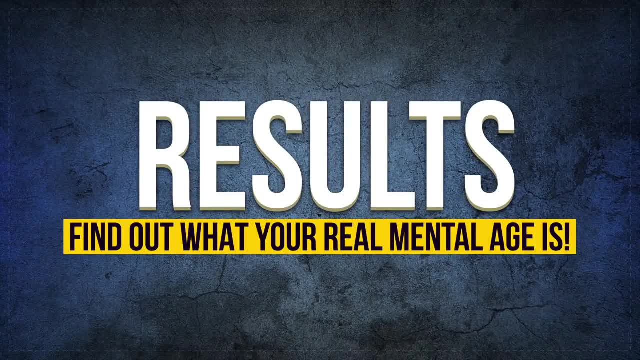 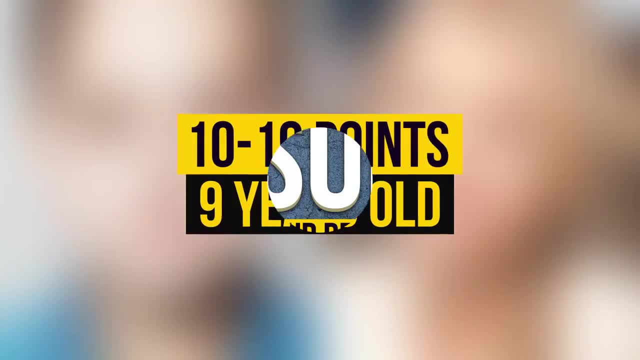 And we are done with the test. Ready to find out the results, Then do your math and find out what your real mental age is: 10 to 19 points, 9 years old. If you got 10 points, 9 years old. 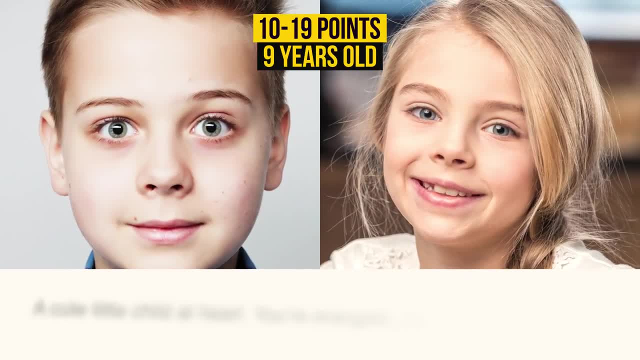 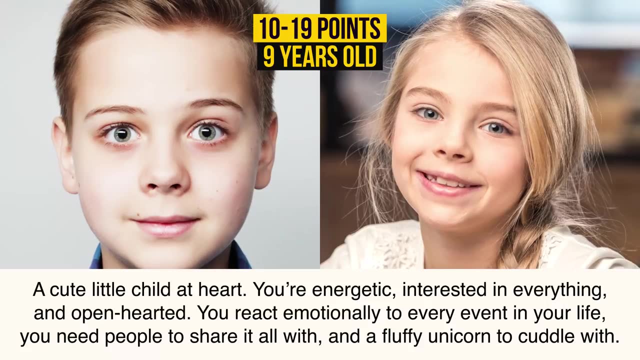 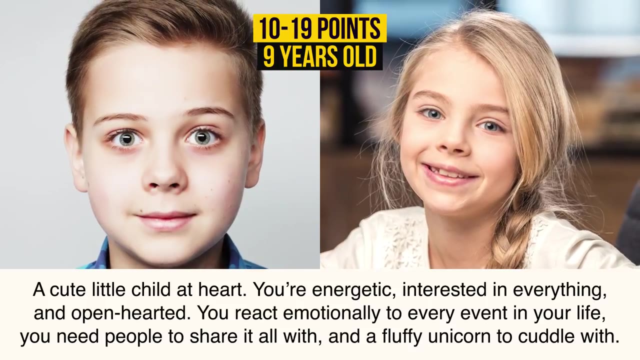 If you got 10 to 19 points. you are a 9-year-old, A cute little child at heart. You're energetic, interested in everything and open-hearted. You react emotionally to every event in your life. You need people to share it all with and a fluffy unicorn to cuddle with. 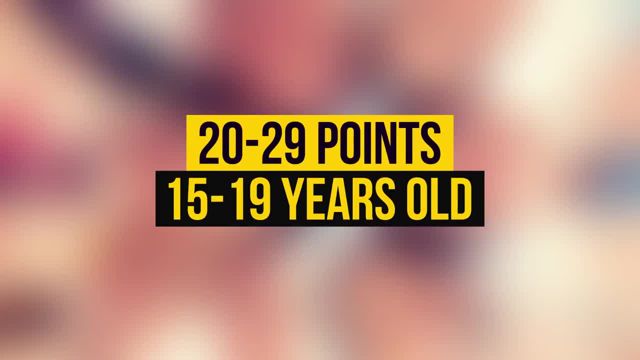 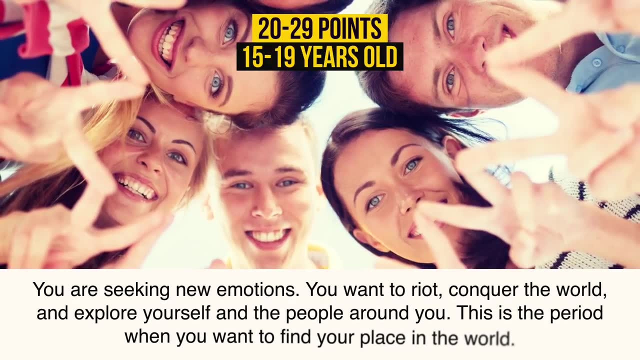 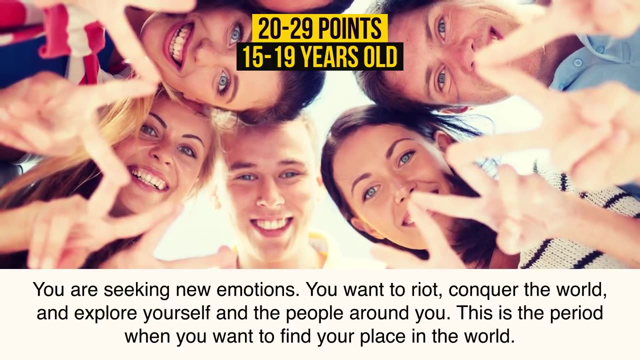 20 to 29 points. 15 to 19 years old. Hello there, teenage soul, You are seeking new options. You want to riot, conquer the world and explore yourself and the people around you. This is the period when you want to find your place in the world. 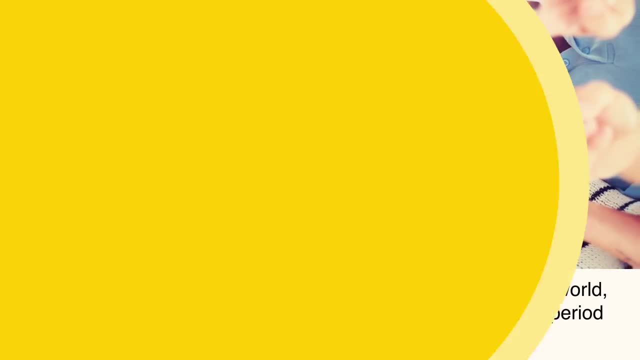 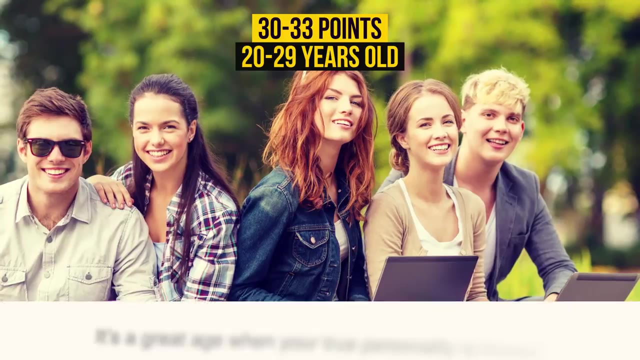 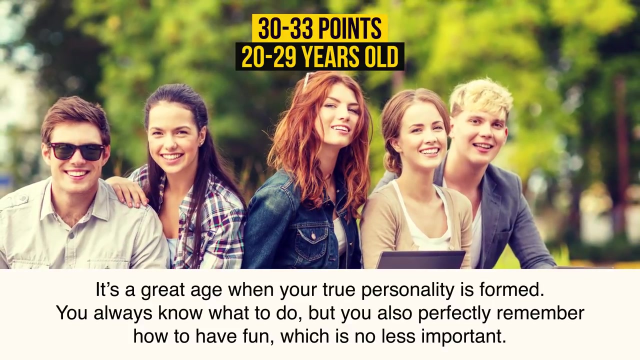 30 to 33 points. 20 to 29 years old: It's a great age when your true personality is formed. You always know what to do, but you also perfectly remember how to have fun, which is no less important, right. 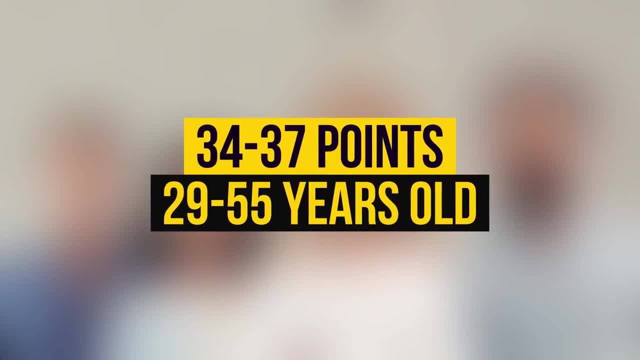 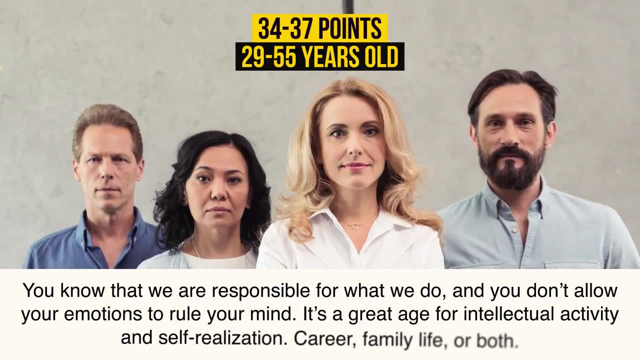 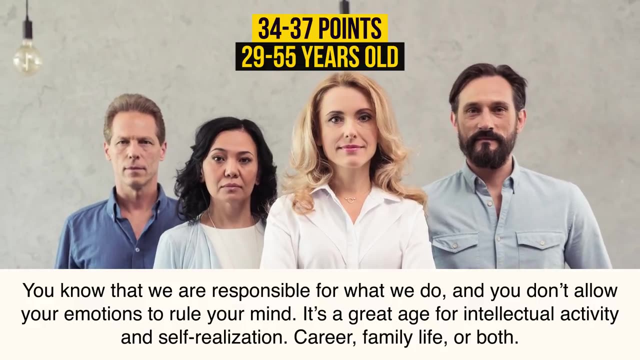 34 to 37 points, 29 to 55 years old. Your mind level is middle-aged, You know that we are responsible for what we do and you don't allow your emotions to rule your mind. It's a great age for intellectual activity and self-realization. 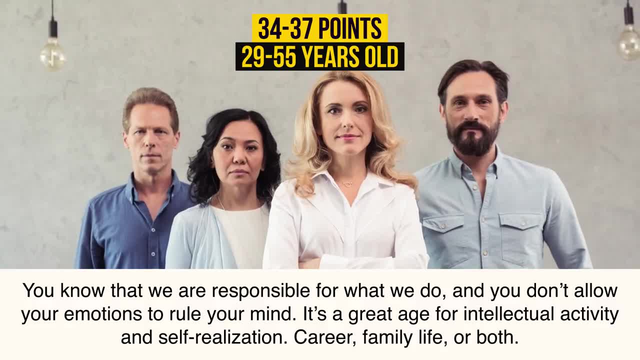 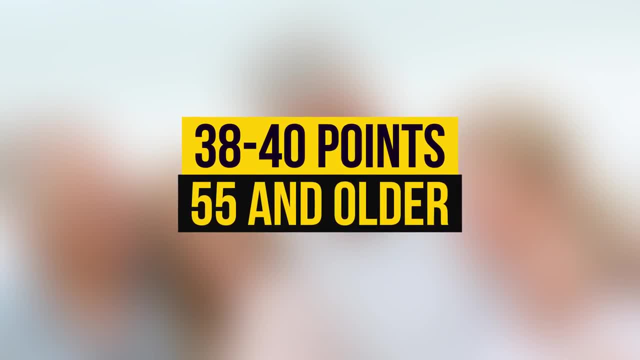 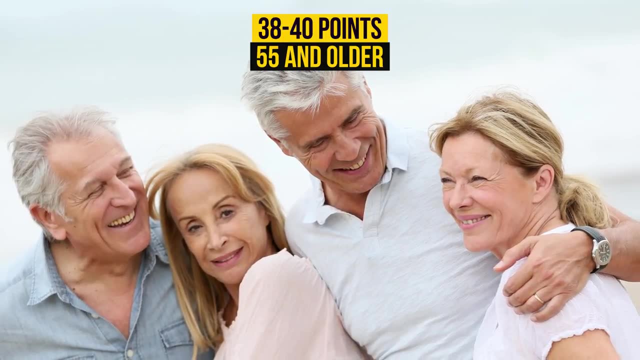 Career, family life or both. this is your time to shine. 30 to 40 points, 55 and older: The age of stability, when you don't have to prove anything to anyone and know how to live for yourself. You wear no mask and always stay yourself. 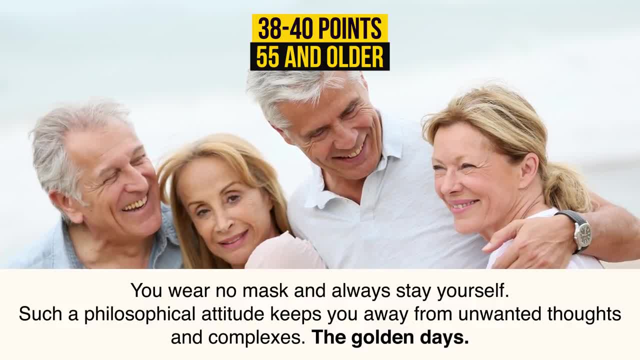 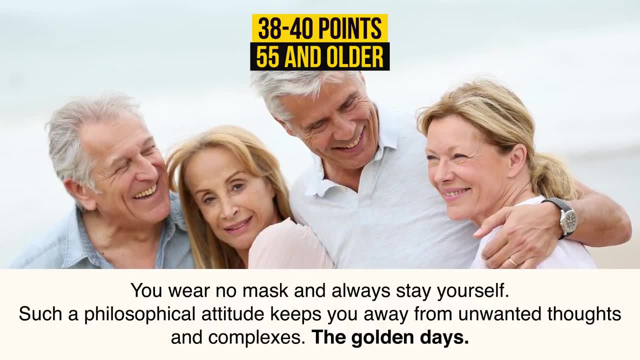 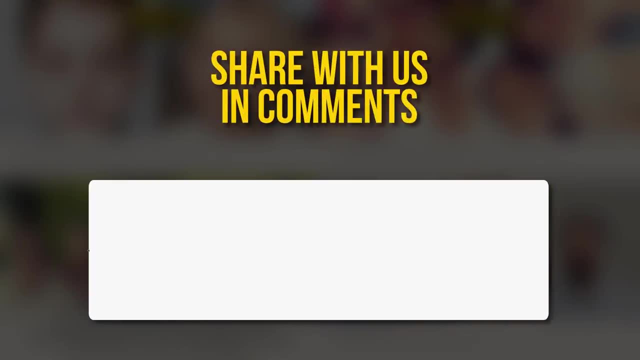 Such a philosophical attitude keeps you away from unwanted thoughts and complexes The golden days Now. are you happy with your results? Do you find them accurate? We have a whole comment section to discuss the test. Feel free to do it. Finally, remember this nugget of wisdom: